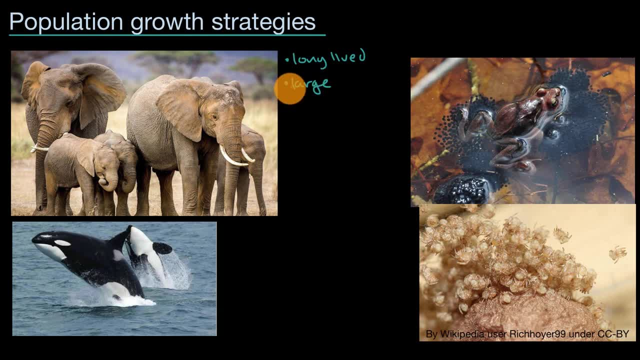 They tend to well, they tend to be large. They- especially if you think about compared to very small things in the animal kingdom- they tend to not have a lot of children. every reproductive event- I guess you could say it- every time they give birth. 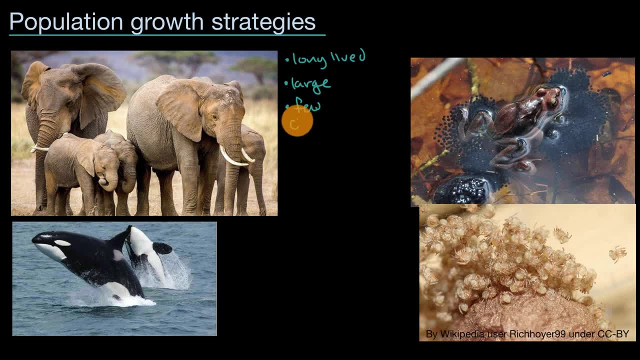 So few, few children, children at a time, And it takes them a while to give birth to those children and then they take care of them for a while. Now, the other end of the spectrum, you have some of the things that we have here. 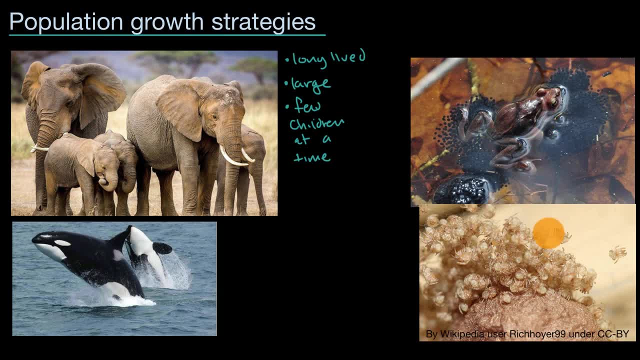 You have amphibians like frogs, You have insects- You could imagine small fish, bacteria, mosquitoes that are more short-lived, Short-lived, Short-lived They have. they tend to be smaller And they tend to have a lot of children at a time. 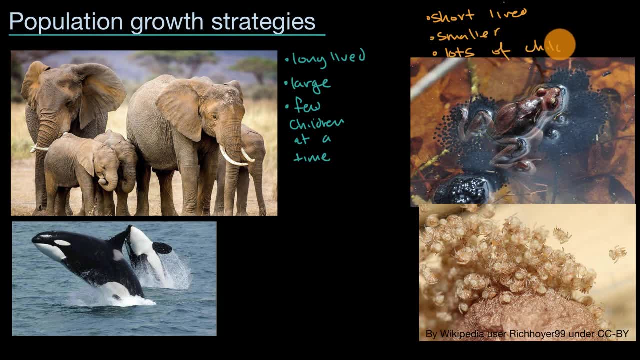 So lots of children at a time. Just an example: a frog or what you see here is this is spiders coming out of an egg sac. Frogs, or spiders, they can lay, you know, they can lay eggs. They can lay eggs. 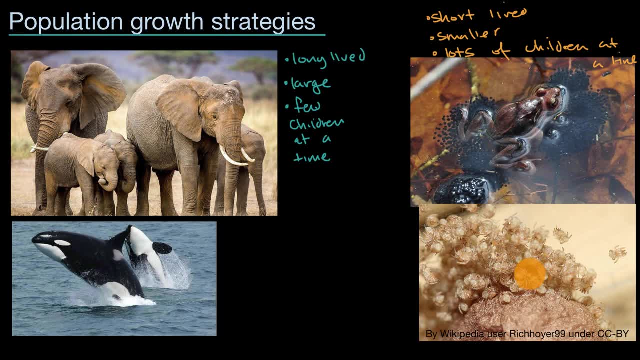 They can lay in many cases thousands of eggs at a time And they're not really dependent on any one of those eggs necessarily surviving. Many of them will be killed off by predators, But as long as a few survive, then the next generation you can imagine. 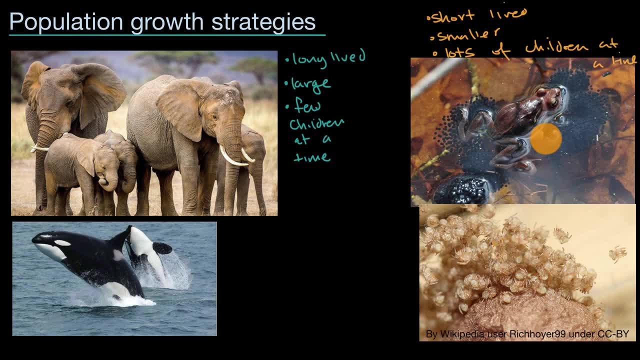 they get to reproduction and then they'll lay thousands of eggs And they're shorter-lived: A frog could live a few years. Some insects might live anywhere from a few days to a few years. You have things like bacteria that can have an even shorter lifespan. 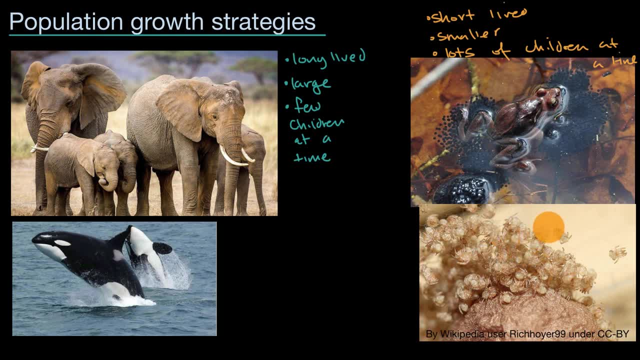 So when biologists or ecologists look at this, they say it looks like there is a spectrum over here. You have these large, long-lived animals that have a few children at a time And really the limiting factor on their population is how dense their population is. 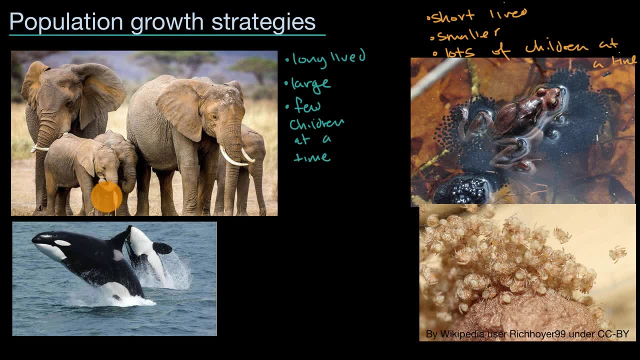 At some point, these animals are going to compete for resources with each other, And that's true of things like human beings. At the other end, you have these things like spiders or frogs, and they're going to compete for resources with each other. 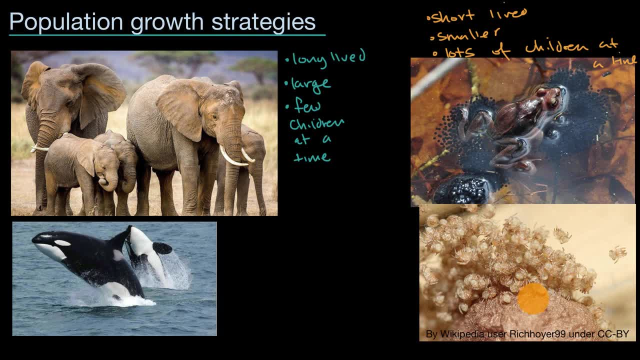 Instead, they might be limited on their reproduction by environmental factors like how moist or dry it is, how hot or cold it is, And so, generally speaking, folks have attempted to classify these types of species. They call them K-selected, and I'll talk about where the K comes from in a second. 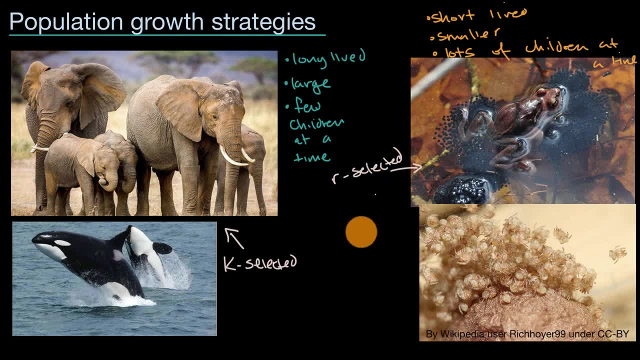 And they talk about these types of species as R-selected. And where these letters come from is that there's a general idea that if we draw a little axis here- time- and then draw an axis here- population on the vertical axis. 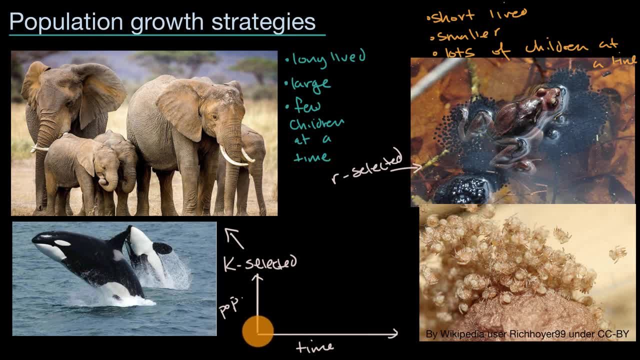 most species that when there's not a lot of them and they're not limited by resources, they will grow exponentially, like this. Now, when you go into the math of it, that rate of growth is usually denoted by the letter R. 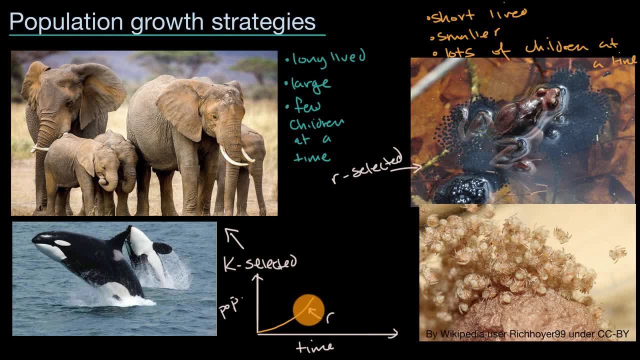 and you could see where this R-selected is coming from And what that R is. how large it is is determined by a species biotomy and it's called biotic potential, And biotic potential just means in a given environment. 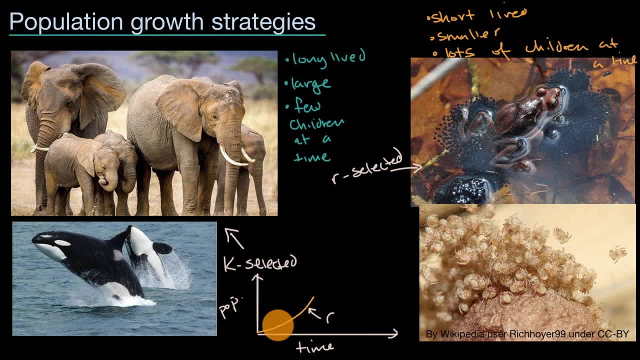 how quickly can they reproduce, what percentage of those are able to get to maturity so that they can reproduce, et cetera, et cetera. And so you could imagine, the higher the R, the faster this exponential growth goes up. 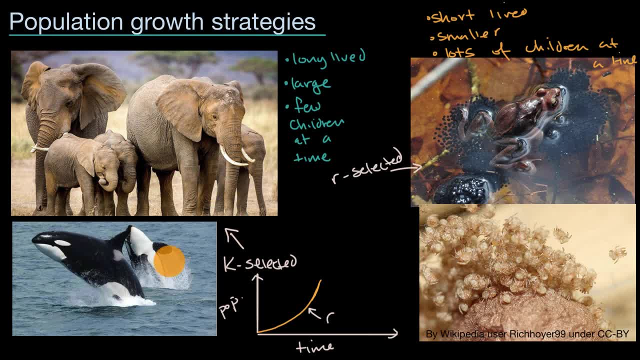 Now, at some point you're going to be resource constrained and there's some carrying capacity, And so let's say: this is the carrying capacity here, and let's call that K. And the reason why we use K instead of C is K comes from A word for capacity in German. 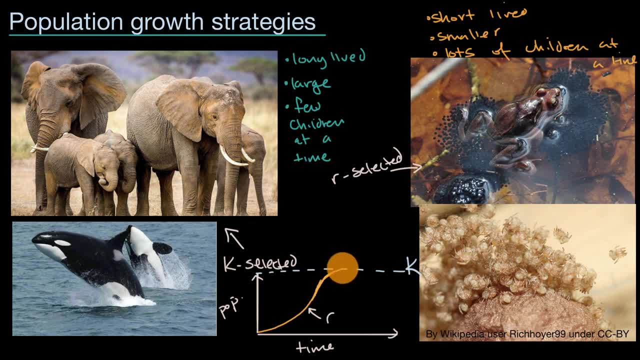 So at some point, you're gonna have so many things that you're just not gonna have enough resources to support more, and so your population would flatten out something like this, And so, generally speaking, biologists have categorized these left categories of species as K-selected. 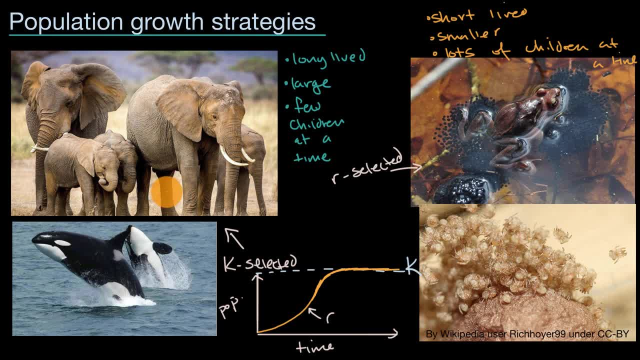 They are the amount that you have. the amount of population is going to be determined by the amount of resources that are there, the carrying capacity in the environment, While things like frogs and mosquitoes and bacteria and spiders you view more as R-selected.